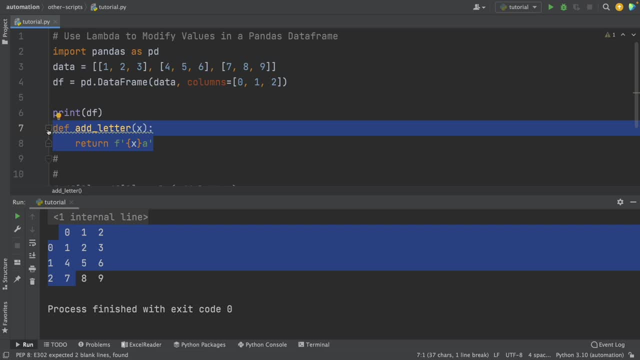 this isn't complicated, but creating functions for every change we need to make in a data frame is not practical. This is when Lambda comes in handy. The Lambda function is similar to the regular Python function, but it can be defined without a name, which makes it a nice. 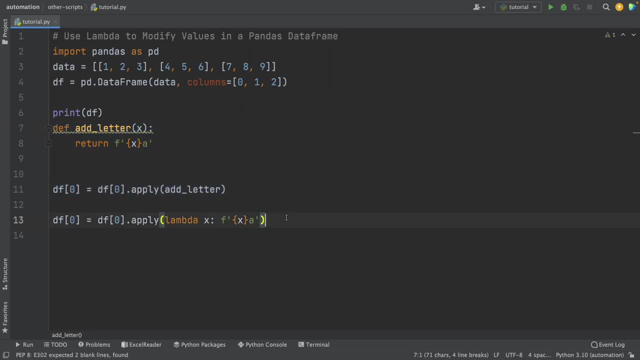 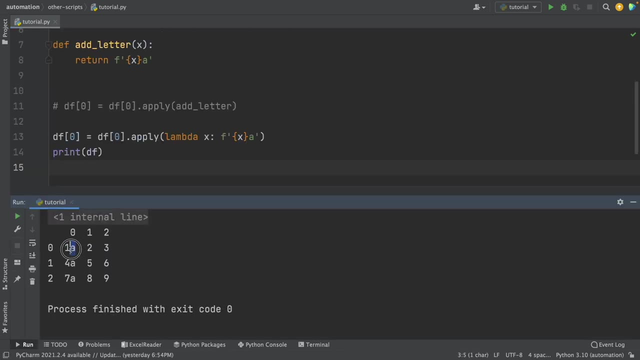 looking one liner. All this code I wrote can be reduced to this single line of code. Now, if I print this data frame after using the Lambda function, you can see that this letter A was added to the values in the column zero. All right, and now another common beginner. 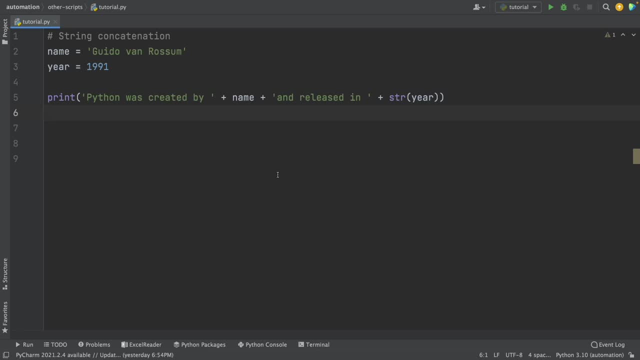 mistake that we make when we learn Python. for that analysis, It's using the plus operator for string concatenation. The most common way to concatenate strings in Python is using the plus operator. However, a big issue with this operator is that the syntax is not so clean and also it cannot go beyond joining strings, For example. 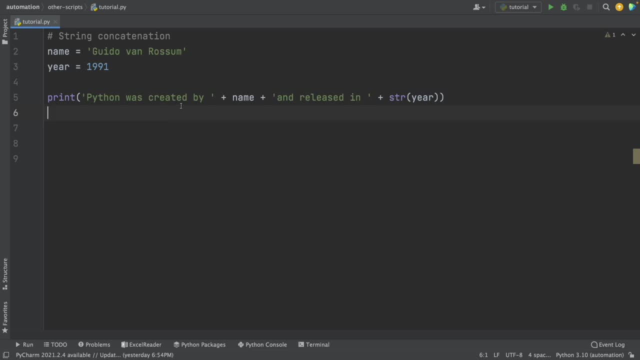 here if you want to create this sentence. Python was created by Gideon Rusin and released in 1991.. You have to convert this year variable, which is an integer, into a string to build this sentence. In contrast, F strings work in the same way. If you want to create this sentence, you have to 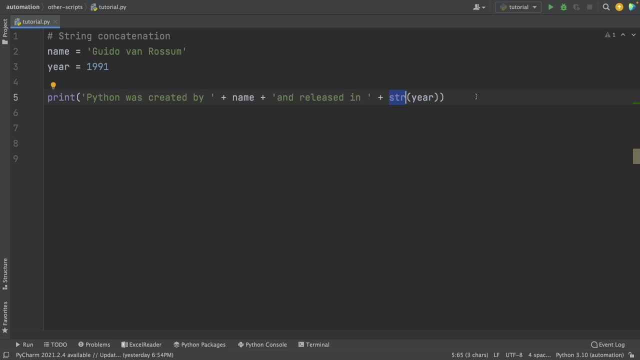 use curly braces to store a value that will be formatted into a string. If we rewrite this into an F string, we'll get this. So now the syntax is cleaner. We can see Python was created by, then the name and released in and then the year, And we don't have to use the str function to turn. 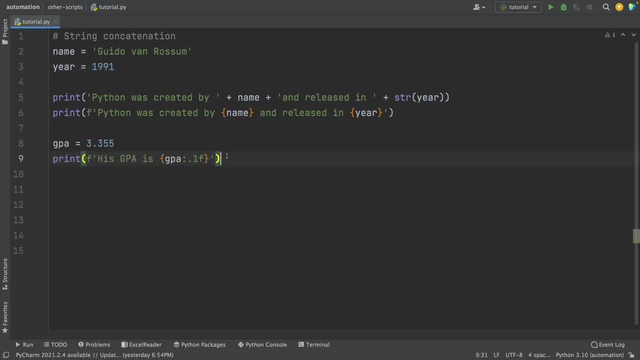 this integer into a string, but this is done automatically. Another advantage of the F string is that you can customize how the string is going to be printed. For example, here I have this part which I'm going to use. I will say: print gpa equal to 3.355.. And here, if I want to print: 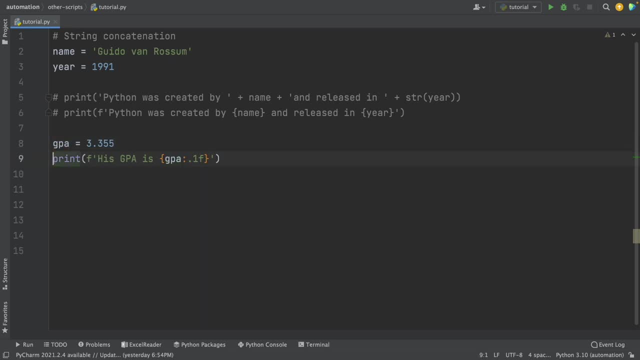 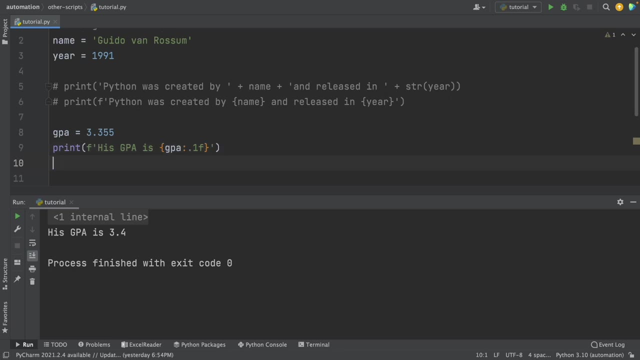 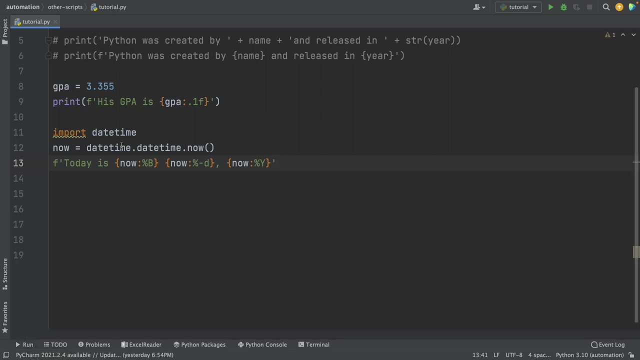 his GPA is, and then use only the first decimal of this value. I can use this .1F, which indicates that I want to round this to the first decimal. And also you can do other things, like using special functions inside the F string. For example, here I'm going to use the daytime function. 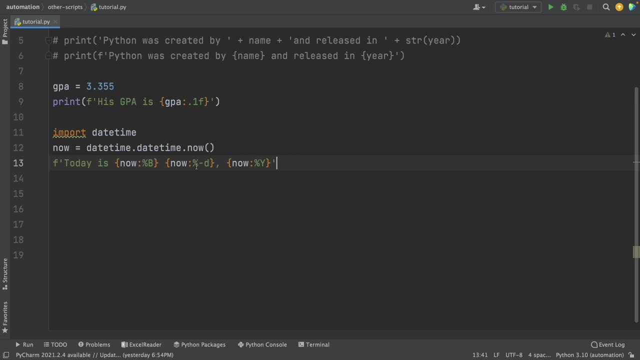 to print today's date. So here I import the time And now I use the percentage B, percentage D and y to get the year, the month and the day of today's date. So here you can see: if I print this I'm going to get today's date. So today is April 9th, 2024.. And now a common mistake we have when 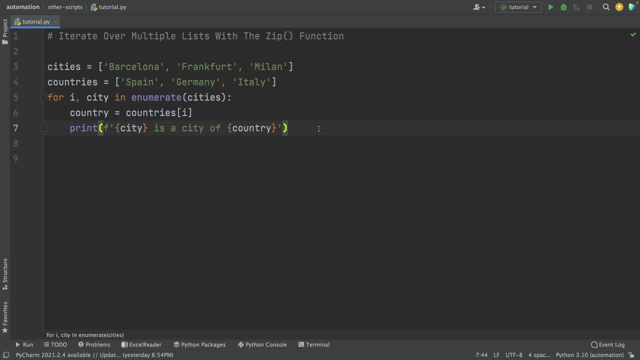 we work with multiple lists is that we want to loop through this multiple list using the enumerate function. This is fine when you have two lists. For example, here I have two lists and I can print this message without any problem. A better way to do this is using the zip function. The zip. 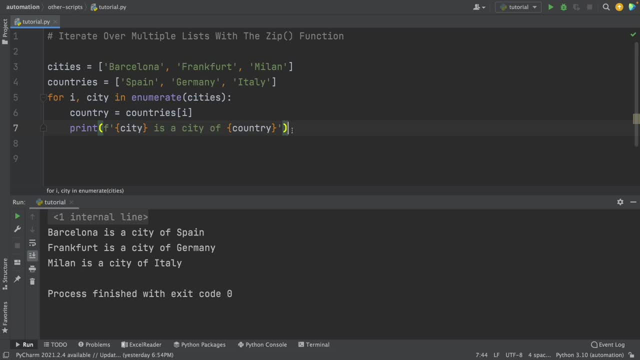 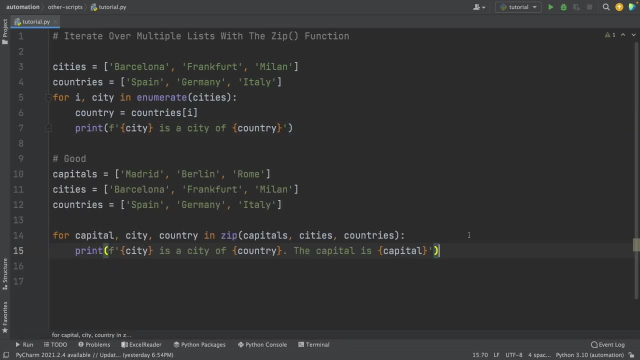 function takes iterables, aggregates them in a tuple and returns it. Let's see how we can print a similar message, but now with three lists. Now here I can loop through the three lists and build this message that you can see here: Barcelona is the city of Spain and the capital is Madrid, And the 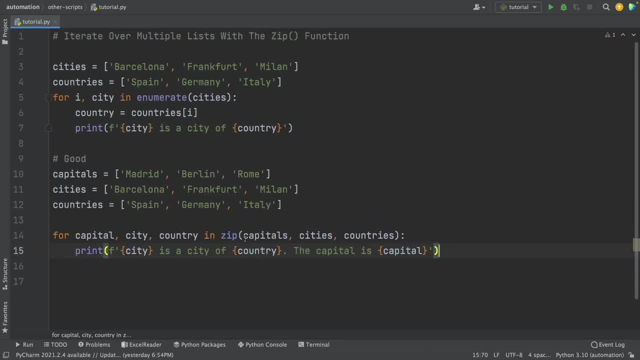 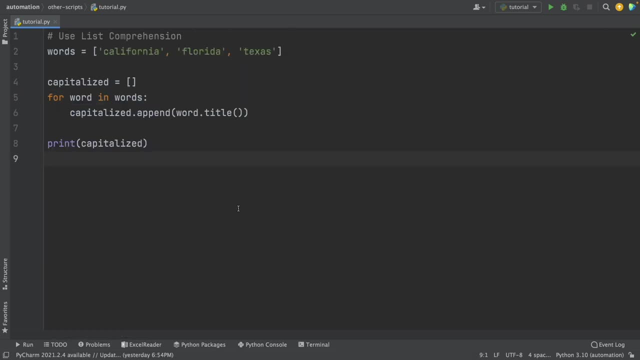 other two sentences as well, And I could do this using the zip function, And this would have been more complex if I had to do it in a different way, So I'm going to do it in a different way. Use that enumerate function, All right. another common mistake we use when working with data. 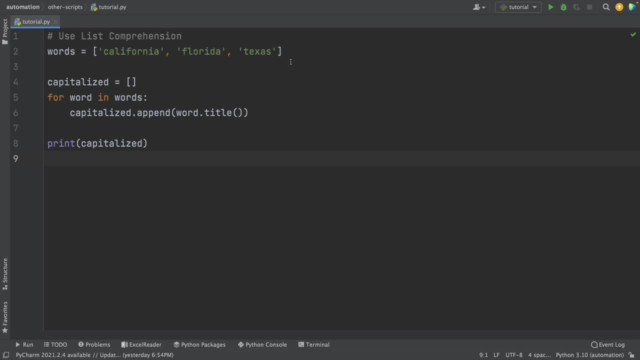 is not using list comprehensions. For example, here I have a list that I named words and this has the states of the USA, So California, Florida and Texas. And if I want to capitalize this, sometimes what we usually do is creating an empty list and then using a for loop to modify every. 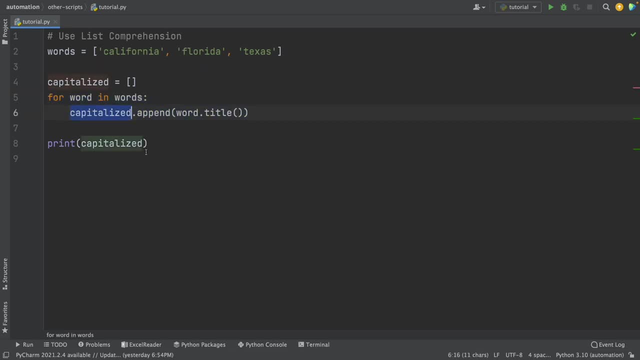 value of the list And then append this to the empty list. So here, if I print this, we get the job done and it's just going to be a list. And then, if I print this, we get the job done and it's just going to be a list. And then, if I print this, we get the job done and it's just going to. 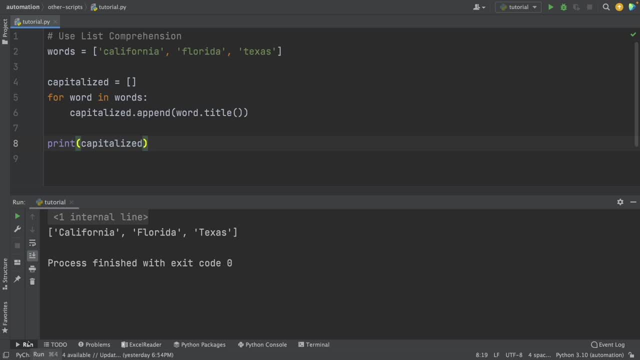 be a list, And then, if I print this, we get the job done and it's just going to be a list. As you can see here, the values of the words list are capitalized. There is nothing wrong with doing this, But something much better to do is using list comprehensions, And I'm going to show you. 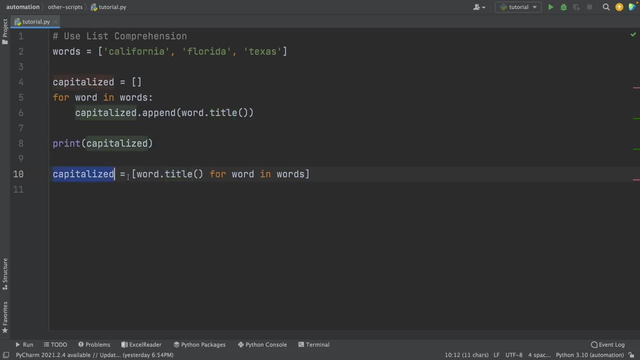 how this works And what we do here is creating a list And inside this list we do the for loop. So here you can see for word in words, And then on the left you see the action that we want to make in the elements of the words list, In this case wordtitle. So we want to capitalize. 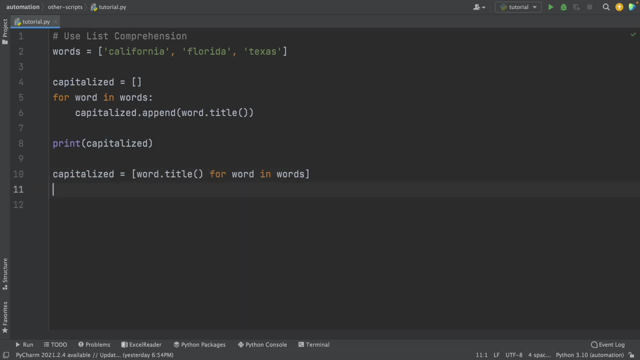 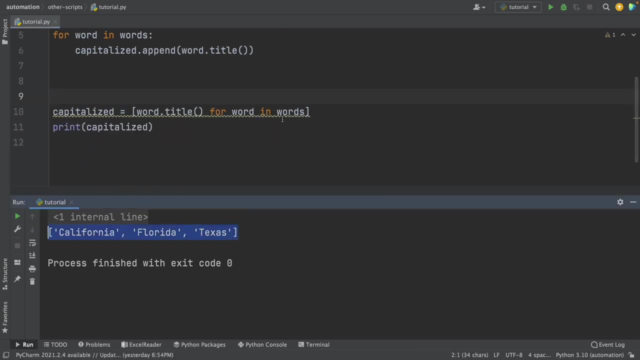 every element of the words list. So now, if I print this, this capitalize list, Now I'm going to get the same result, but now using list comprehensions, And this is sometimes more practical than doing all of this, Alright. another common mistake we often do when 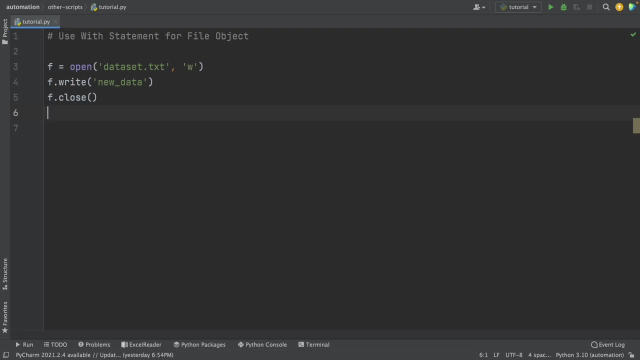 working with file objects, as a data analyst is not using the with statement. So, for example, here I'm reading a file using the open function And what we usually forget to do is use the close that I wrote before and I just delete it, And well, that's easy to remember. but sometimes after 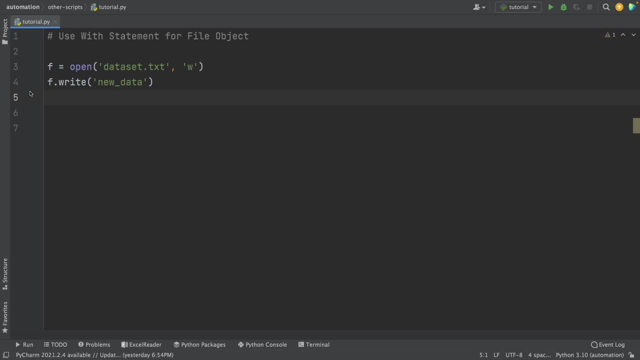 writing code for hours, we might forget to close the f file, And this is when the with statement comes in handy. The with statement will close the file object automatically. And here is how it works: You only have to use with, then the, the function, the open function here, and you have to read it as: 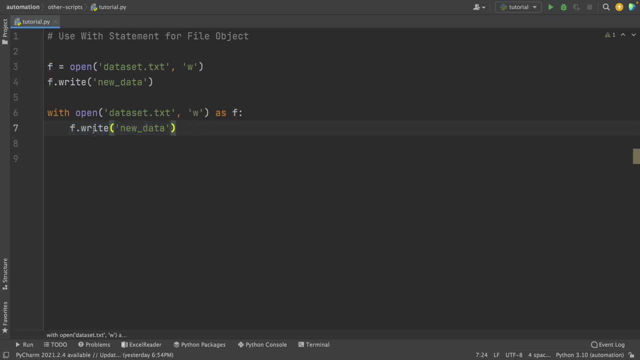 f, And then you do the action below, And well, in this case I want to write new data, And that's how you do Here. you don't have to write the f that close that we tend to forget, But only use that with statement. And I use this with statement to write the file object. And then you have to 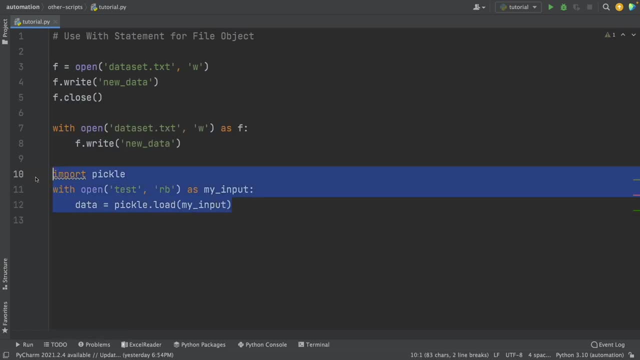 write the statement very often when I pickle objects, as you can see here, because I don't have to close the file manually, as I showed you before. Alright, we often make the next mistake when collecting data for our data analysis project. Say, we're scraping a website, So here I'm importing. 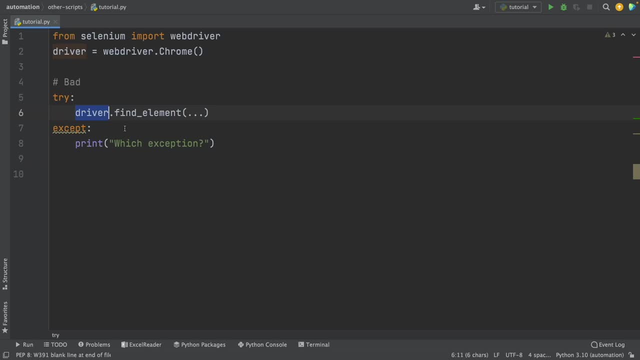 WebDriver from Selenium And then I'm trying to find an element using the driver. And here a common bad practice we make is using the try except, but only using a bear accept. The problem with a bear accept is that it will catch system exit and keyboard interrupt exceptions. And also, when you read the script it's not completely. 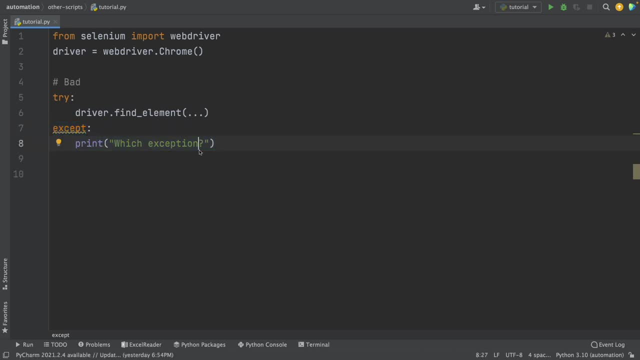 understandable what exception you want to catch here. So it's a better practice to specify the exception in the except clause And if you're using Selenium you only have to import the exceptions. For example here: no such element exception and element click intercepted exception. 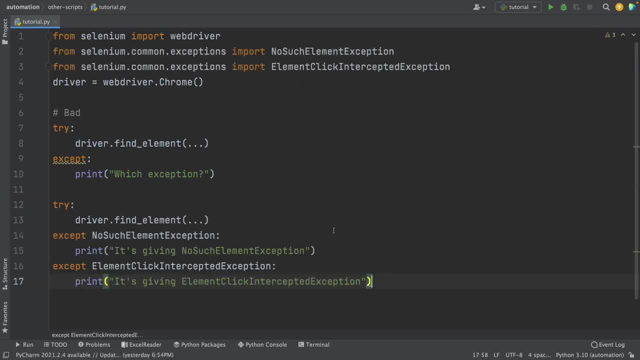 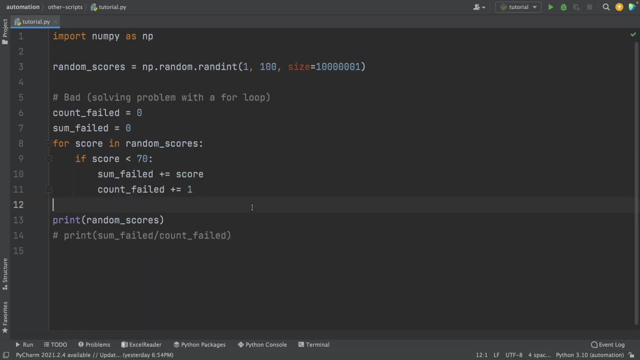 And then you have to add them to the except block. So here you can add multiple except blocks for each exception, And this is more readable and you will avoid the problems that I explained before. Here's another mistake that we often make, And this is overusing the for loop. Often we forget that there are packages that can make. 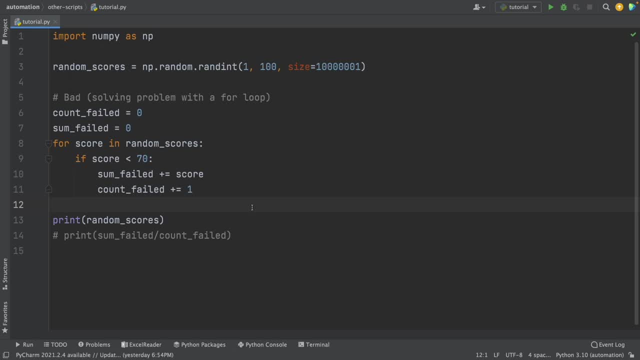 our life easier. One of those packages you should use as a data analyst is NumPy. NumPy could help you solve math operations faster than for loops. Say, we have an array of random scores and we want to get the average score of those who failed the exam, So I score less than 70.. 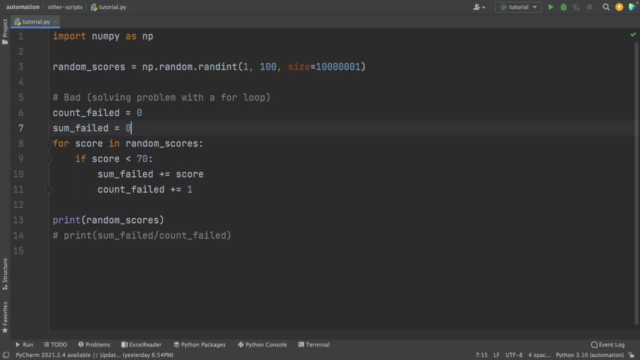 Let's try to solve this with a for loop. If you try to solve this with a for loop, you will have to create these two variables and then use this for with this if condition. So here you sum the scores of those who failed the exam and divide it by the number of. 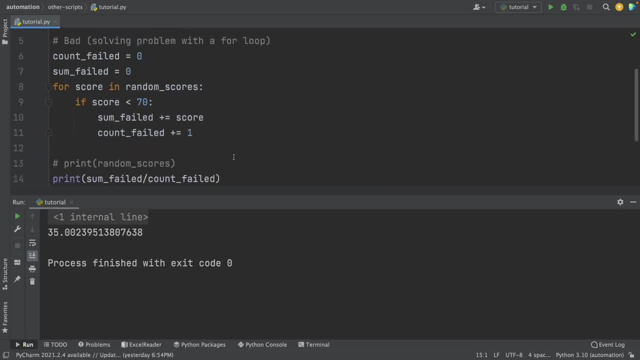 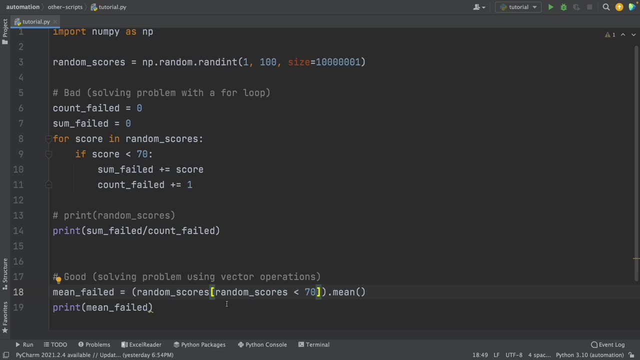 people that failed the exam And you get the answer of this problem. But you can simplify all of this for loop using NumPy. So instead of doing all of this, you can simply use NumPy vector operations to filter those scores that are less than 70 and then to calculate the mean. 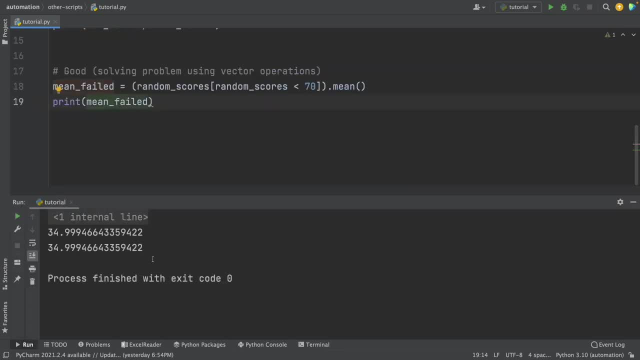 And that's how you get the same answer- using NumPy. And another reason to use NumPy is that it's way faster than doing a for loop. Another mistake that we make when we're beginners is not using the keys and values methods properly when working with dictionaries. And in case you 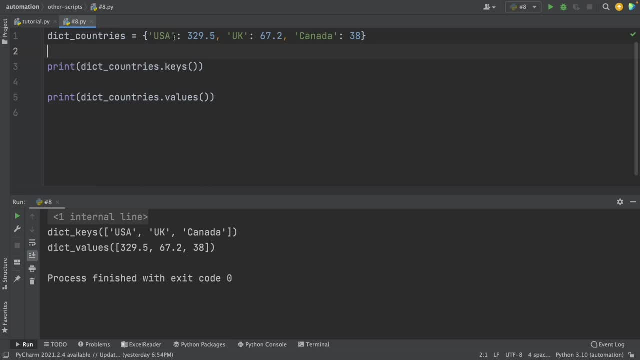 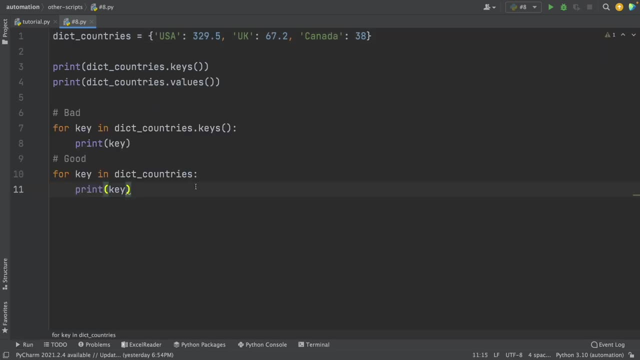 don't know the difference between keys and values in a dictionary. here those in green are keys and those in blue are values, And the problem here is that we sometimes don't use them properly. So you want to loop through the dictionary and obtain the keys. You might use the keys method, as I'm doing. 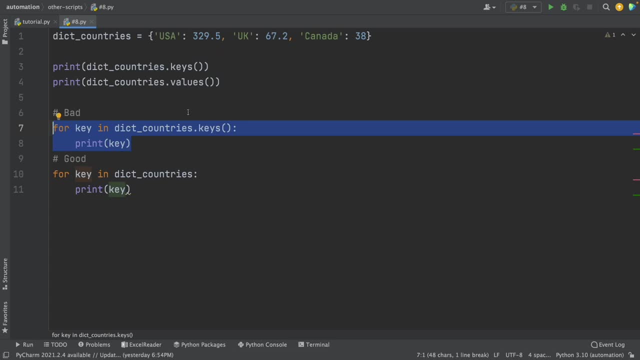 here in this first example. But did you know that you could obtain the keys just by looping through the dictionary, as I showed you in the second example? If I run this, you will see that I will get the keys in both examples. Also, we might come up with workarounds to get values for a dictionary. 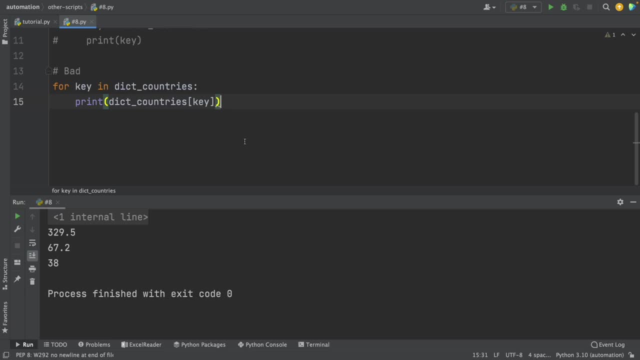 as I showed you in this new example, But that could be easily obtained with the items method. So don't forget to use the items function to easily obtain the keys and values of a dictionary. Alright, before I continue with these common beginner mistakes, remember that there are many. 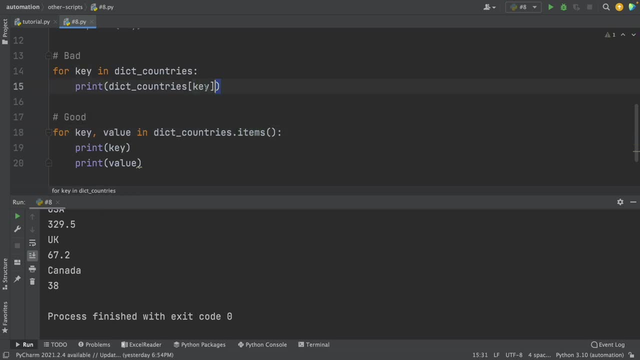 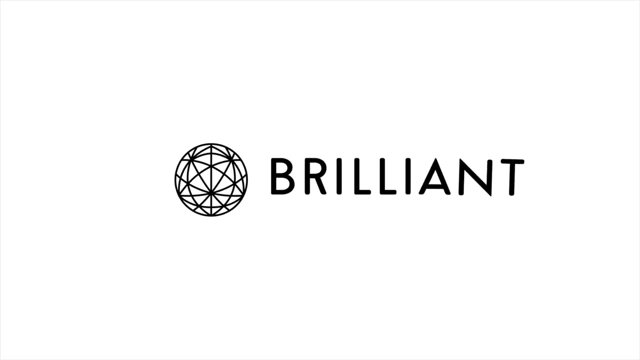 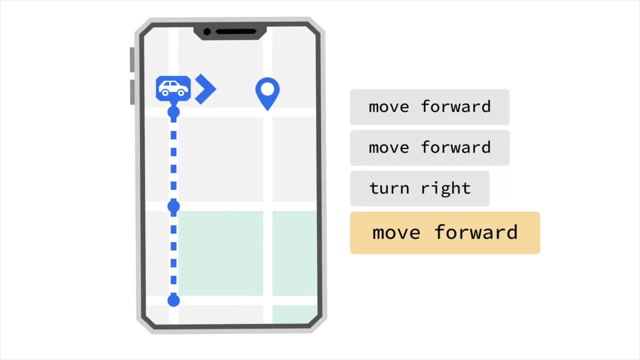 other mistakes not included in this list. If you want to avoid them all, what I recommend you is to learn to think like a programmer, And that's something today's sponsor, Brilliantorg, can help you learn by doing With thousands of interactive lessons in math, data analysis, programming and. 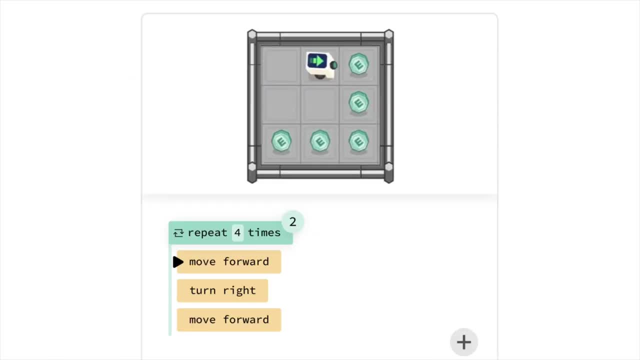 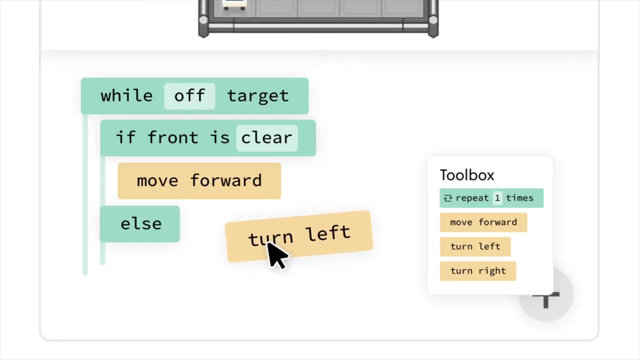 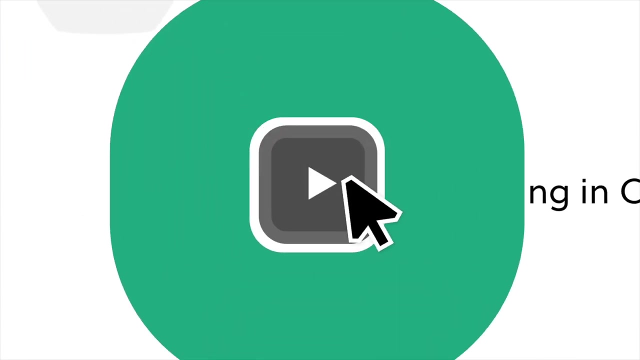 AI Brilliant is a learning platform that helps you build understanding from the ground up. Each lesson is filled with hands-on problem solving that lets you play with concepts, which is proven to be more effective than just watching videos. Brilliant has a section dedicated to Python. It. 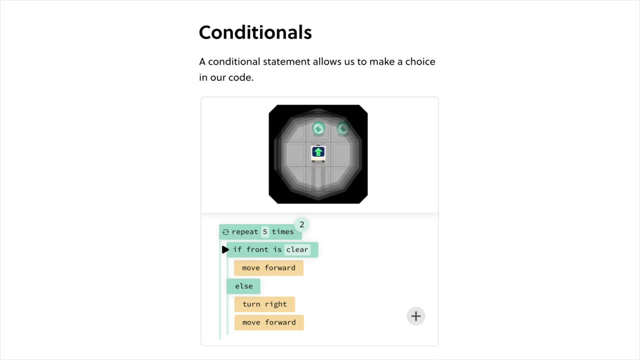 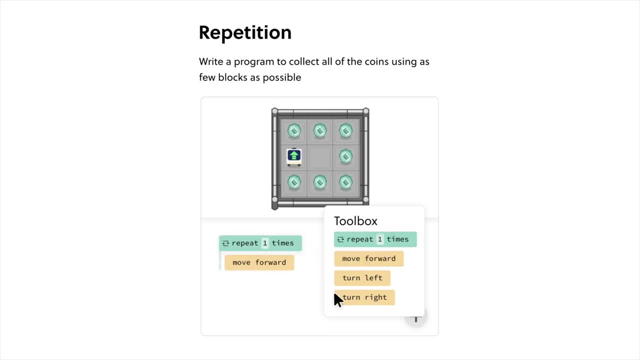 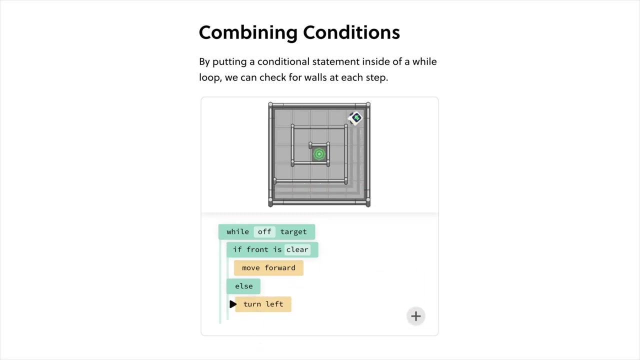 will teach you key code concepts such as loops, variables, nesting and conditionals, Allow you to learn programs on day one with a built-in drag and drop editor and, most importantly, develop your mind to think like a programmer, which is better than just memorizing programming concepts To. 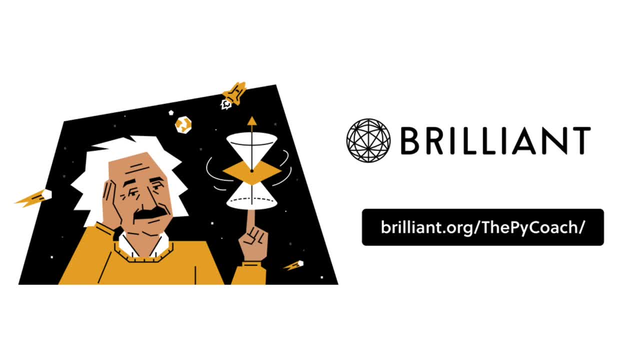 try everything Brilliant has to offer for free for a full 30 days. visit brilliantorg, slash the pycoach or click on the link in the description. You'll also get 20% off an annual premium subscription. Thanks to Brilliant for sponsoring this video. and now let's go back to the video. Another common 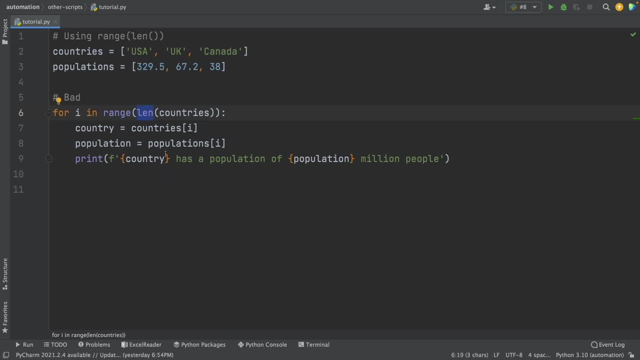 way to learn is using the combination range and length functions to obtain the elements of two lists. For example, here I want to build this sentence using the elements of the country and population list. So I do a for loop and I use this range and length combo and that's how I get. 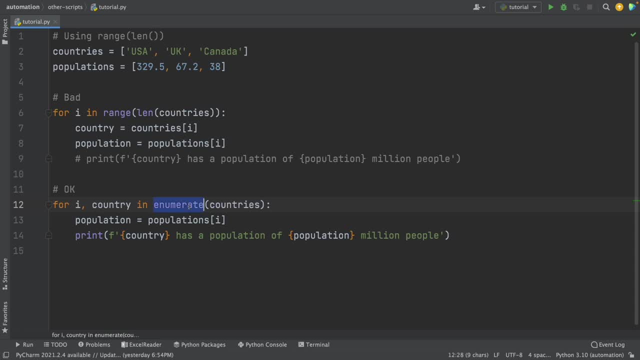 these three sentences, But a simple way to do this is using the numerate function. This replaces the combination of range and length and you will get the same result. And if you want to go to the next level, you can use the zip function. The zip function will help you iterate through multiple 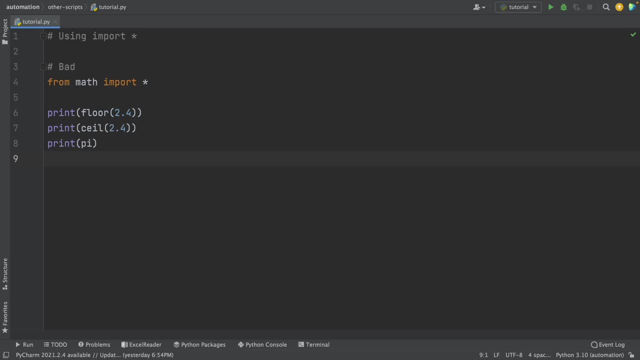 lists and you will get the same result. And finally, a mistake we should never make is importing everything. When we're beginners or when we feel lazy, it's tempting to import everything from a module using the import asterisk. This isn't a good practice because this can be inefficient and 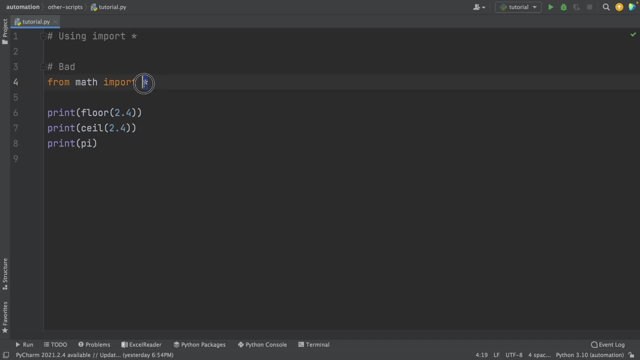 it can cause conflict between variable names. Remember that when you use these asterisks, you don't know which objects you're importing, as well as their names. So instead of importing everything from the module, what you can do is either import the specific object you plan to use or the whole. 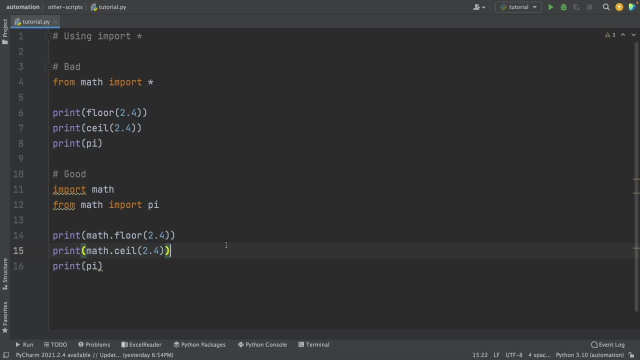 module. In that way, you will avoid different problems in the future. And that's it for this video. Let me know in the comment section what other beginner mistakes you have made as a data analyst or that you know other beginner data analysts have made, and I'll see you on the next video.